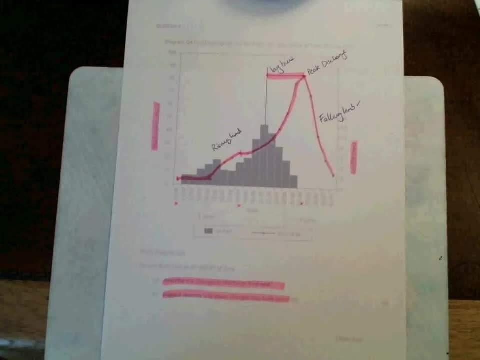 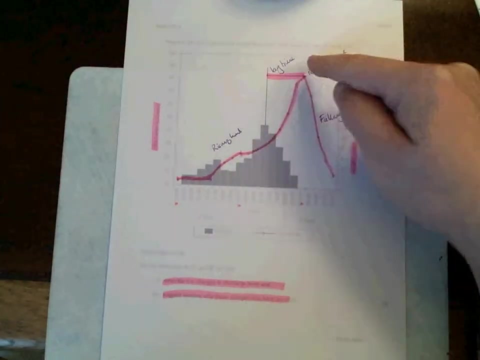 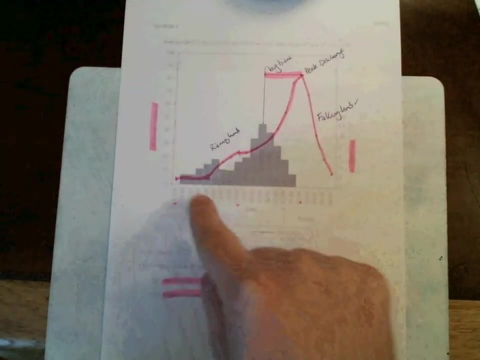 Essentially, what the examiner wants you to do here is to demonstrate your understanding of what factors influence the speed at which the river fills. They have designed the question in order that you can explain why the river is filling rapidly, but also they have actually opened the door for you to maybe be able to explain why some parts the river also was filling more slowly. 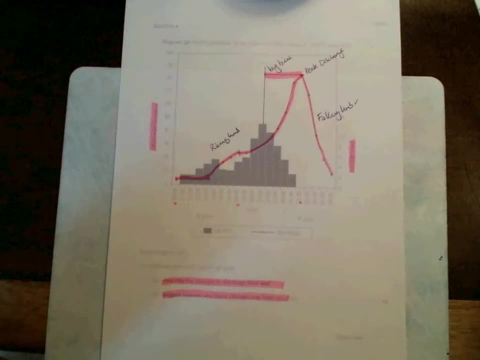 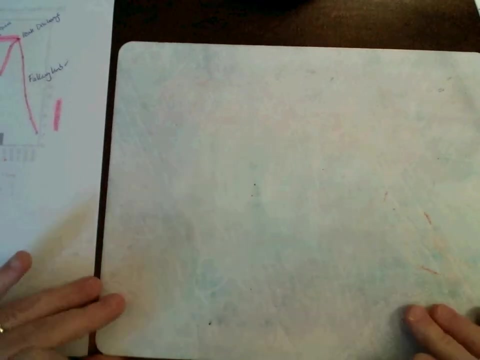 So let's deal with the reasons why the river is filling more rapidly first. I'm a big believer in keeping things simple, And if you want to go through your class notes, you'll see that you've got lots and lots and lots of possible reasons to draw upon. 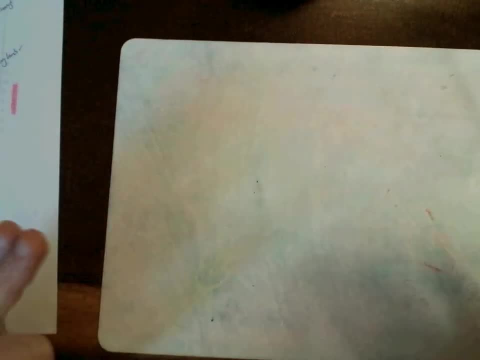 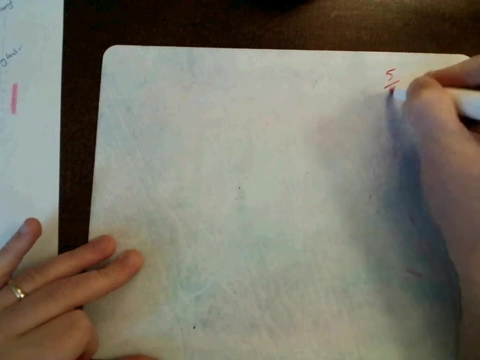 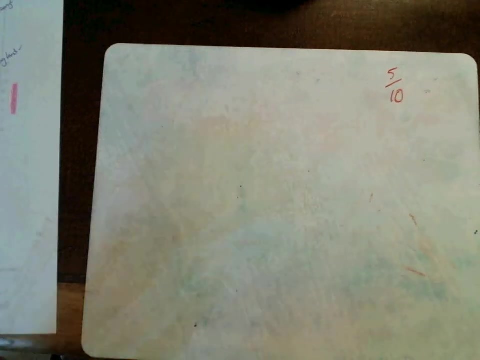 But I want to demonstrate how straightforward this can be. Remember: we've already scored 5 out of 10 for the descriptions that we've done, So now we need a 6 out of 10.. 60%, That's closing in on a B. That's really good. 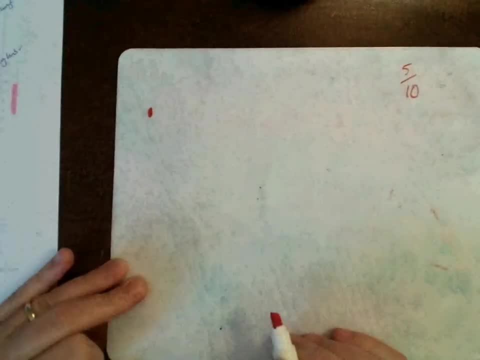 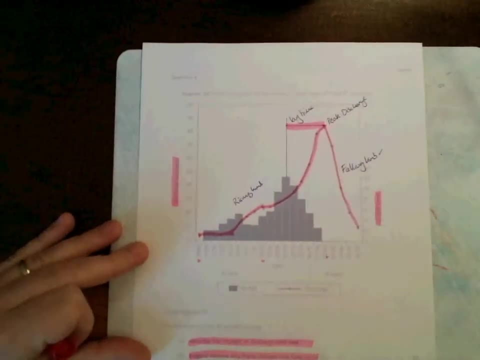 So the first thing that I would point out is that, if we look back at the question, there is nothing in the question that indicates we are not in an urban area. I'll just give you a minute to check that for yourself. 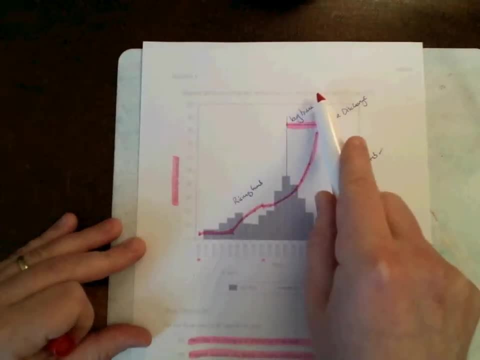 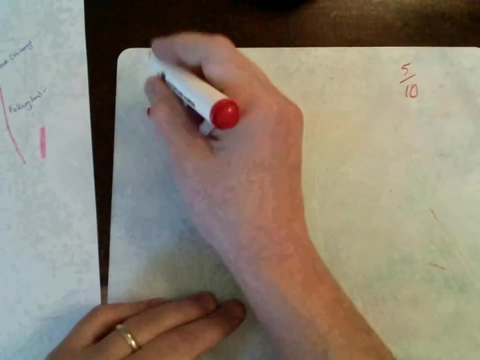 Flood hydrograph at the River Lerry, West Wales, 8th and 9th of June. There's nothing that says it's not an urban area, So I'm immediately going to say could be an urban area. 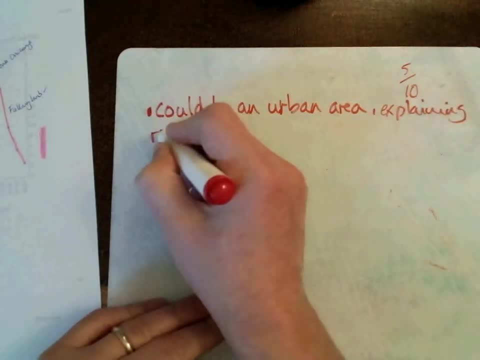 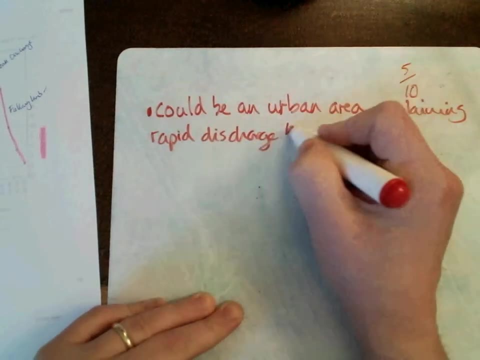 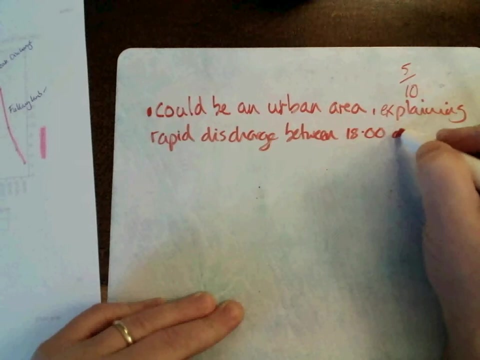 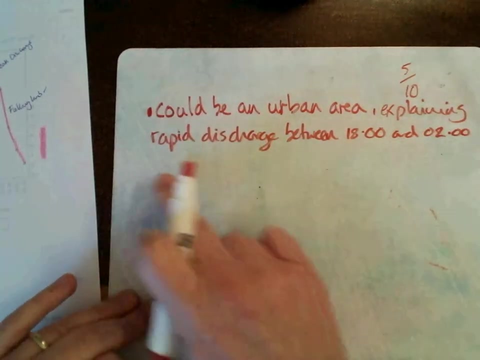 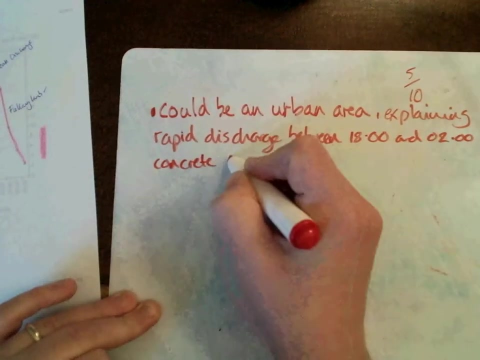 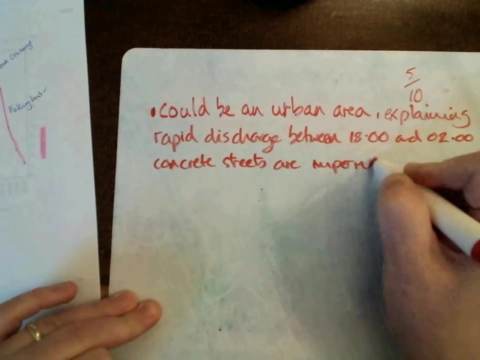 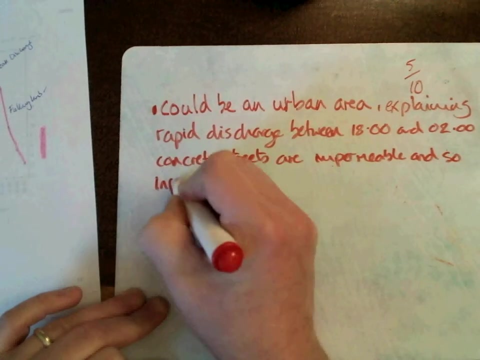 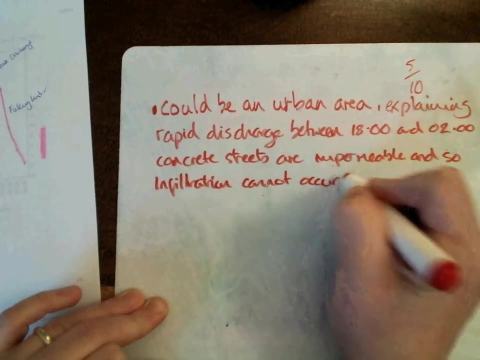 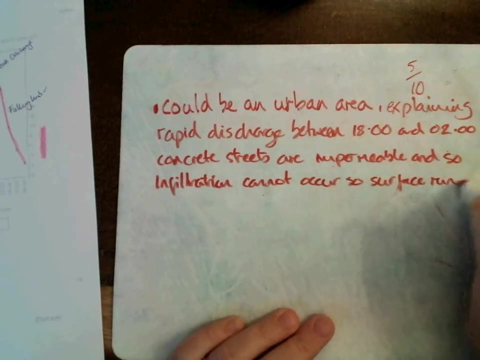 Explaining rapid discharge between 6 o'clock and 2 am, And we need to explain why that's valid. Concrete streets are impermeable And so infiltration cannot occur, So surface runoff is. 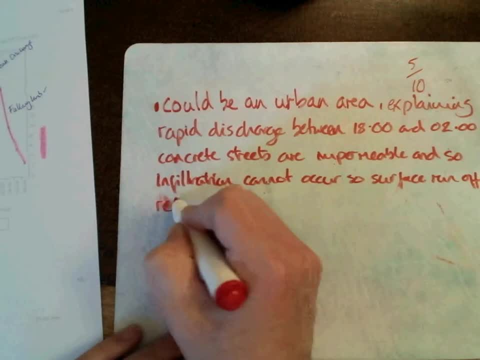 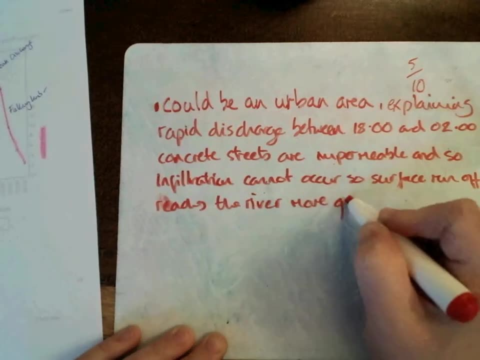 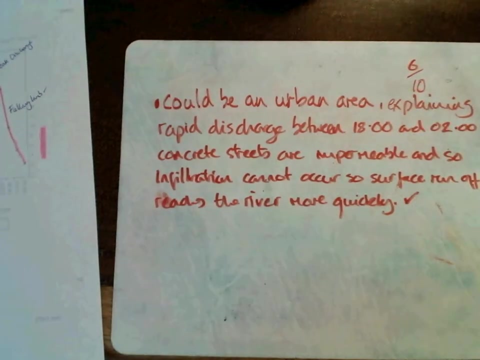 surface runoff reaches the river more quickly. Tick, Immediately, immediately. you're now with just a further little bit of revision and work. we're, we're looking, we're staring at an answer now that we could easily produce an A from quite rapidly. 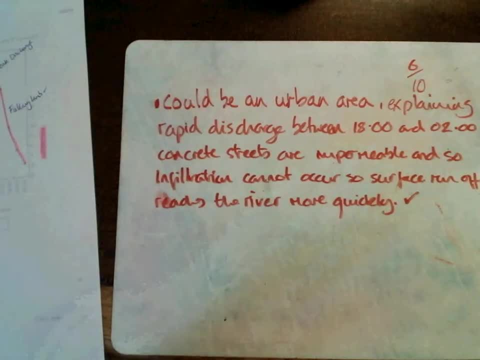 because we've already scored five marks of description. A sixth plus a seventh mark is definitely going to get us up into that bracket where we start to score an A. Why is this a mark is a sensible question for you to be asking. First of all, you've clearly defined what it is that you're explaining. 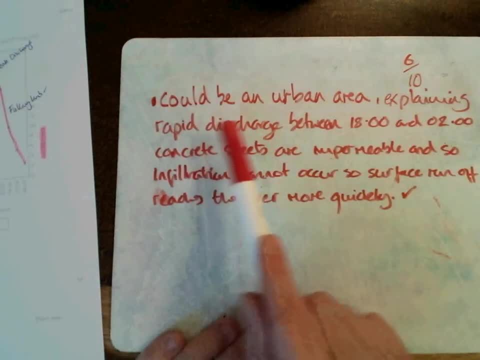 It could be an urban area, which explains the rapid discharge. I'm thinking to myself: where is that rapid discharge? Can you demonstrate that to me? Well, yes, you can. You've said there's rapid discharge between six and two am. 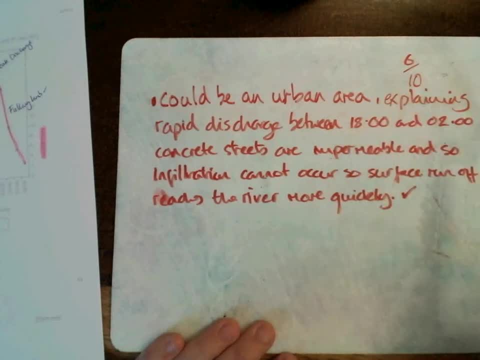 Six o'clock in the evening, sorry, and two am Now. you've probably already pointed that out in your description section of the answer, but it does no harm just to slightly repeat it here Immediately. if you stop there, I'm going to give this symbol and say: 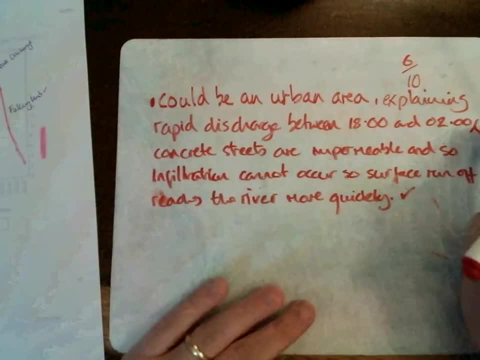 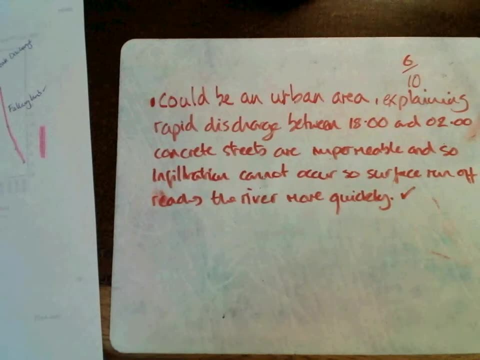 you've not said enough. You you've not developed your point fully. I need to see some understanding of the technical processes at play here. Concrete streets are impermeable. Good A technical term defining a process, And therefore infiltration- another use of a technical term- cannot occur. 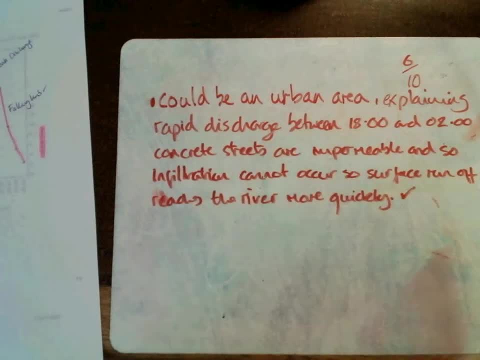 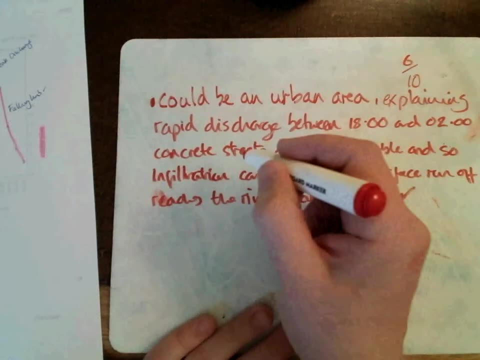 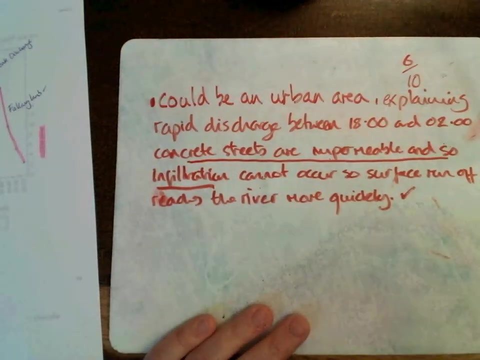 And the impact of this is that surface runoff reaches the river more quickly. Effectively, what I've done is I've said what is happening in this section: Concrete starts to impermeable and infiltration cannot occur, And what is the impact of that? 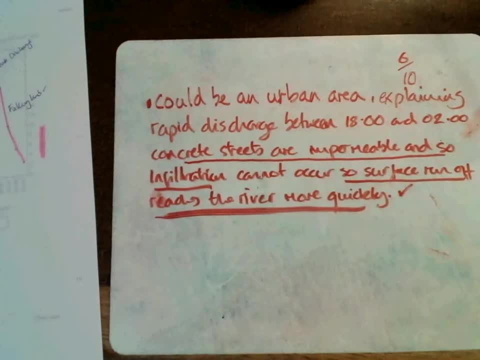 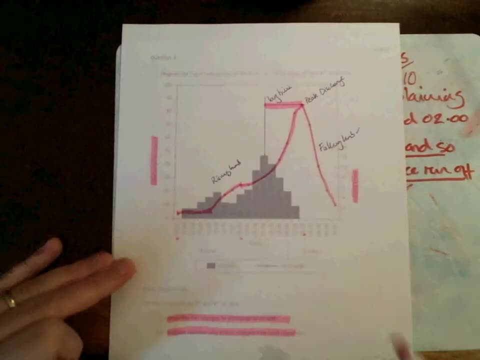 So surface runoff reaches the river more quickly. And there's your mark, And that's us at six out of ten. Just referring back to the question briefly, I'm only concentrating on this area where there's really rapid filling of the river. 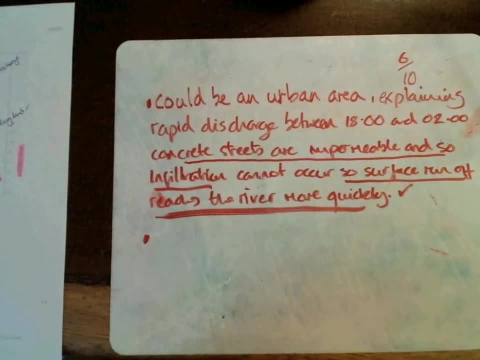 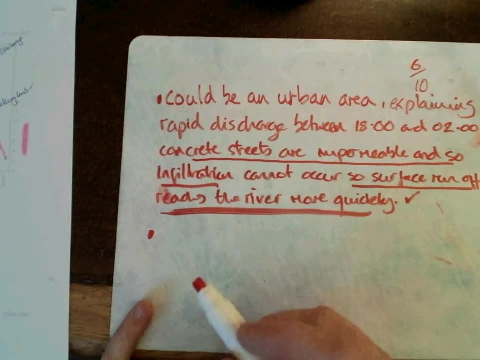 So I'm just going to keep doing that. There's no requirement for me to describe everything that's happening on the river, So I'm just going to concentrate on these reasons why the river is filling rapidly. And again, it's good to keep it simple. 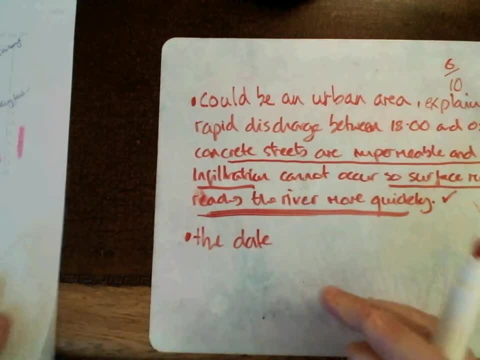 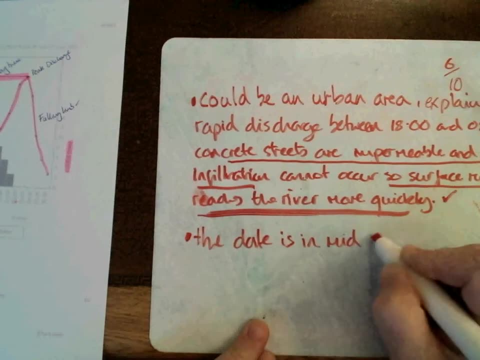 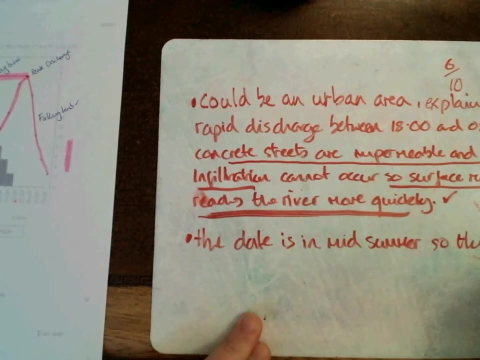 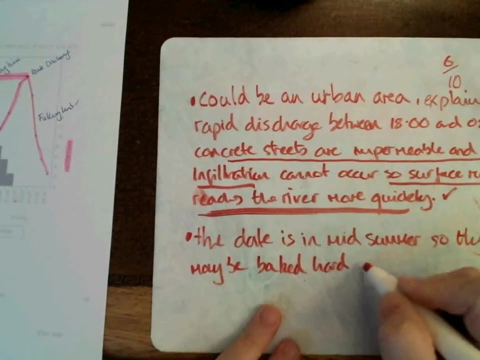 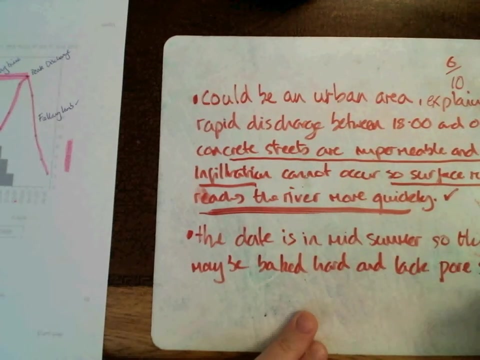 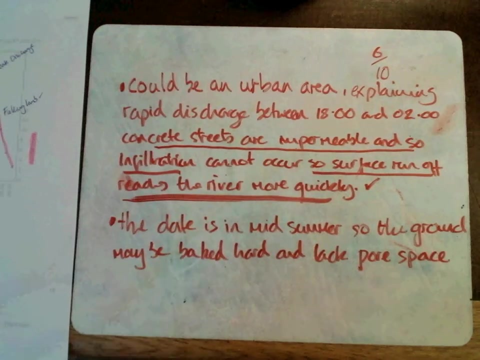 The date is quoted at the top is in mid-summer, So the ground may be baked hard and lack pore space. This is a term you may have forgotten. Pore space means the amount of gaps within the soil for water to infiltrate into. 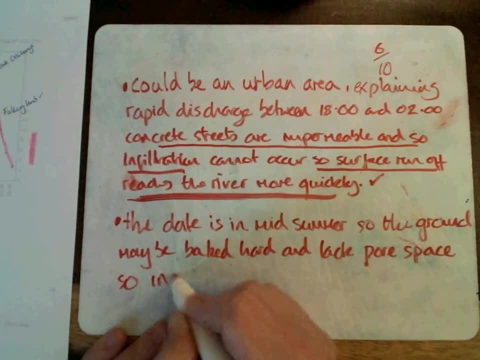 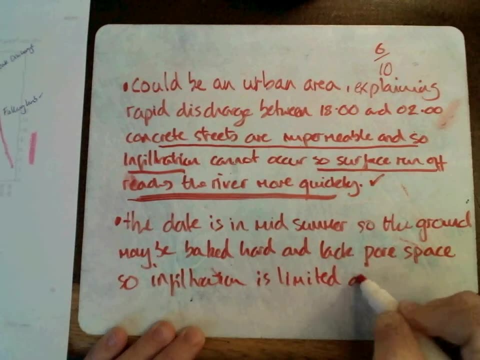 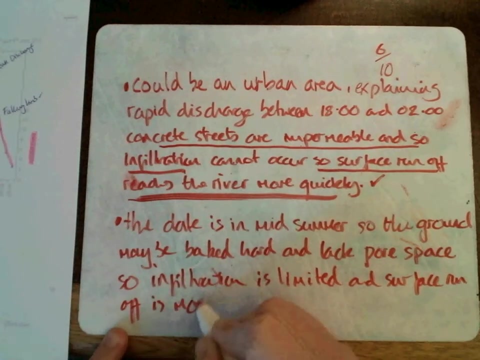 So infiltration is limited And surface runoff is more rapid in reaching the river. The reason I focused on this as an example is because normally- not all the time, but normally- the SQA are kind enough to give you a date in the year. 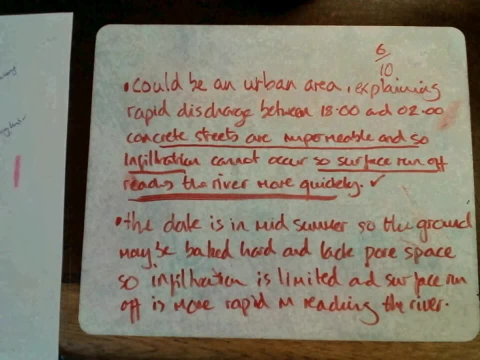 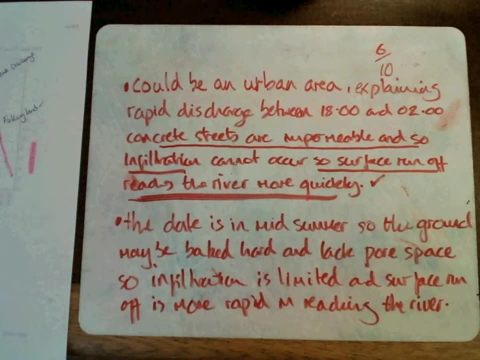 If the date is in winter, well, the ground may be frozen hard And therefore it will be impermeable. If it's in summer, then the ground could be baked hard And this means that it lacks pore space and can be. 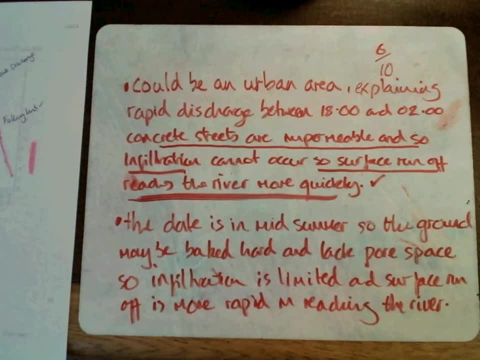 and cannot be infiltrated. Either way, the date is a good way to, in a slightly more easy way, secure yourself some marks. I'm not going to go through every single long and short lag time reason, because we'd be here for quite some time. 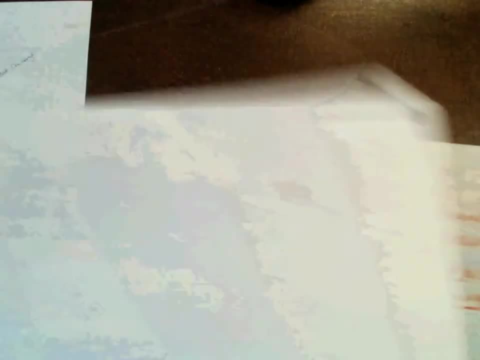 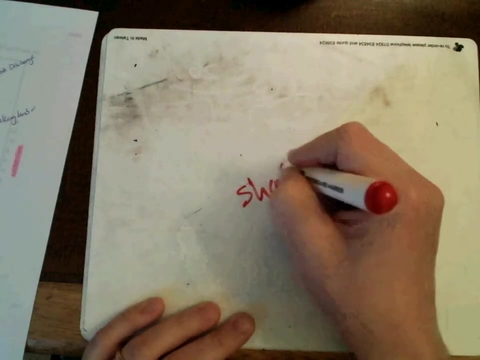 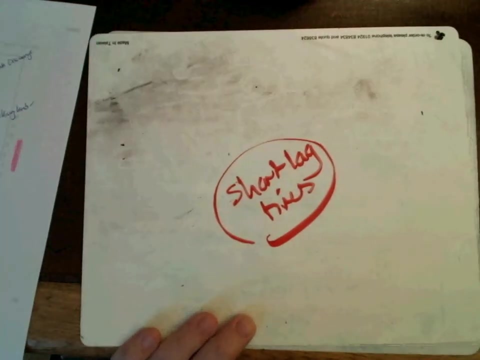 Those are two good ones. What else could you? what else could you? could you talk about, though? Well, for short lag times, the things that I would have revised, and make sure I have an understanding of one. 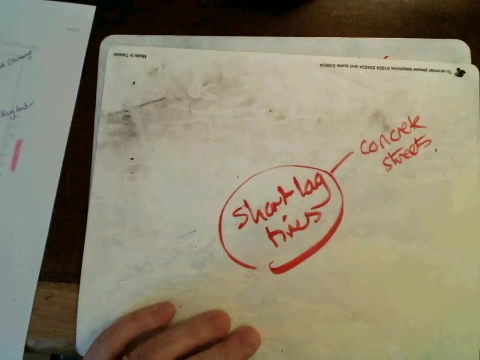 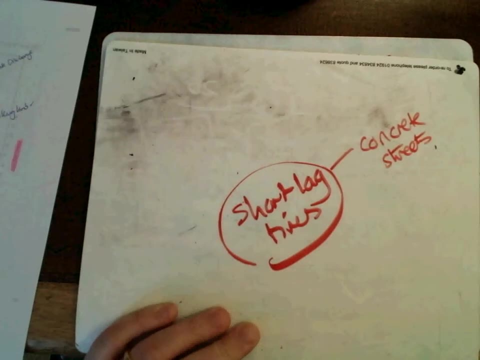 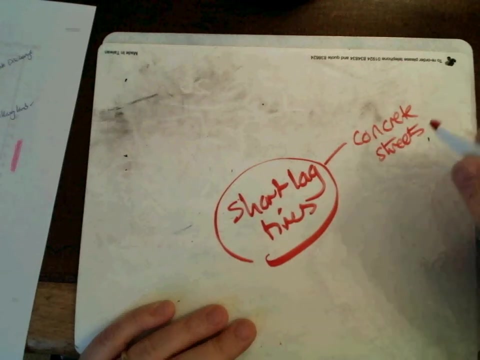 concrete streets. If it's an urban area, then there are concrete streets, And it's just so easy to score a mark with that. Be aware that urban areas don't just have concrete streets, they also have. 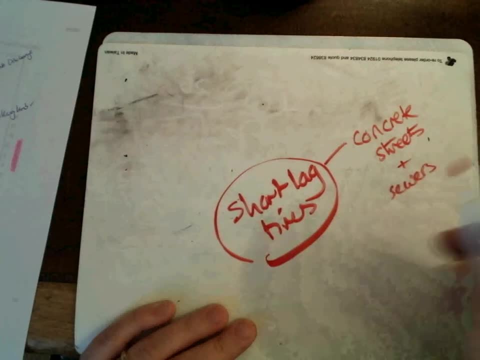 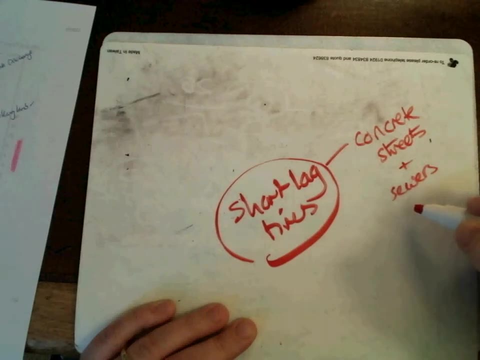 sewers, And sewer systems speed up the movement of through flow, which is an underground movement of water. Both of these things explain rapid increases in discharge. The next thing that I would probably point to is the time of the year. 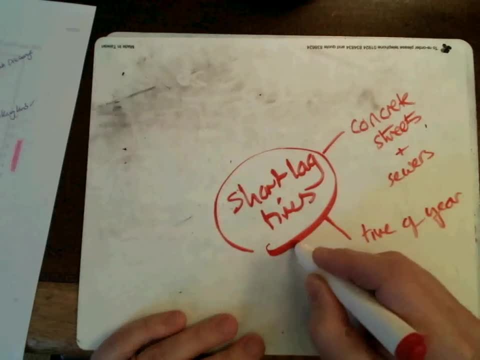 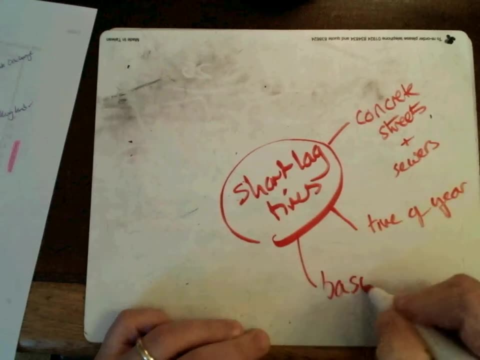 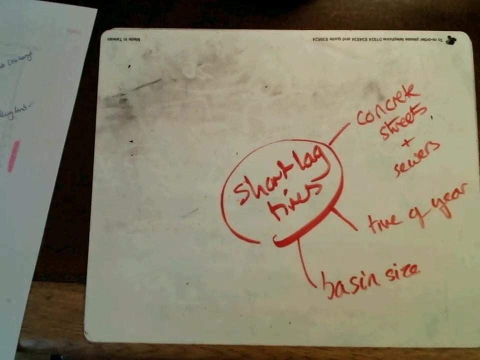 That's nice and easy and I've just explained it. Next up, basin size. If the basin is small, then there's less distance for the surface runoff to travel before it reaches the river. A simple explanation. 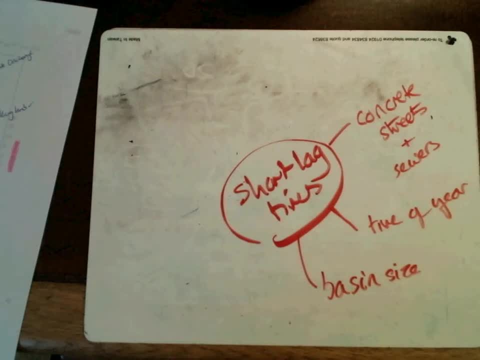 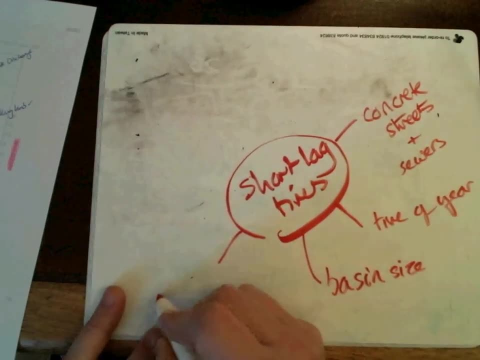 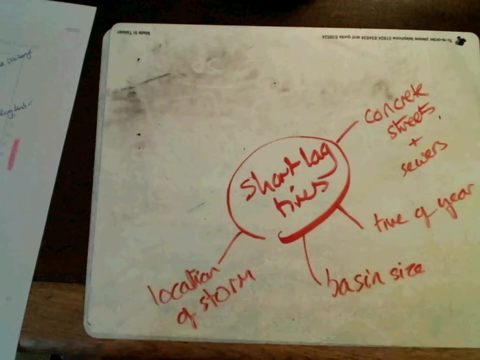 for why the river is filling up quite rapidly. As you'll be aware, weather and storms, they don't just happen in one location, they move, And so it is reasonable to suggest. 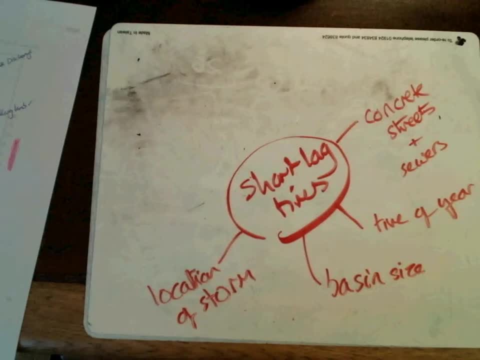 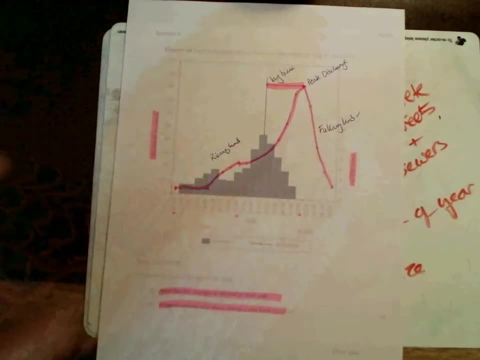 that the storm that took place here's the rainstorm, remember with the bars. this storm was directly overhead over the river and of course that means that the water is going to make its way into the river. 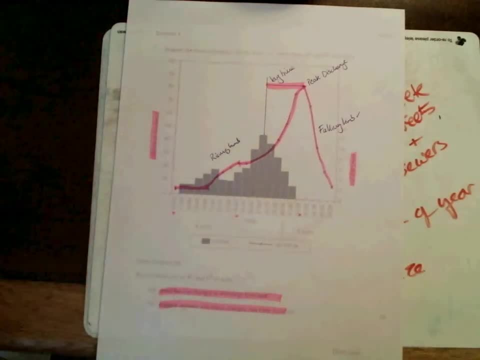 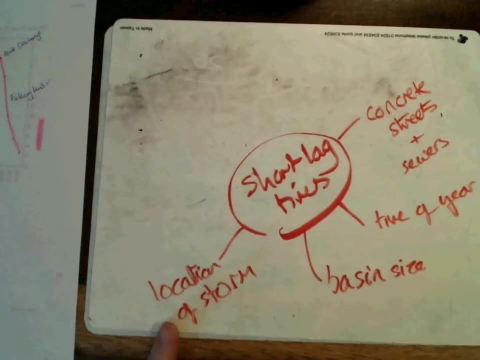 much more rapidly and fill it up more quickly. So the location of the storm is quite important and it's a not an unreasonable and straightforward explanation to offer for why it's so important. The storm was directly overhead. 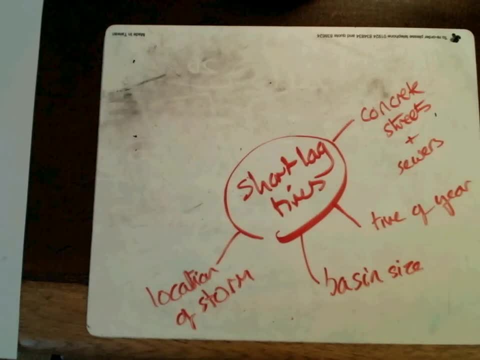 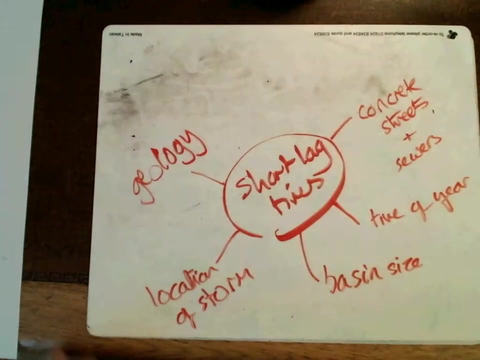 it was over the river, so the water was falling directly into it. Geology: Some people can be put off just by by the word, but really this just means the rocks underneath the ground, and some rocks are impermeable. 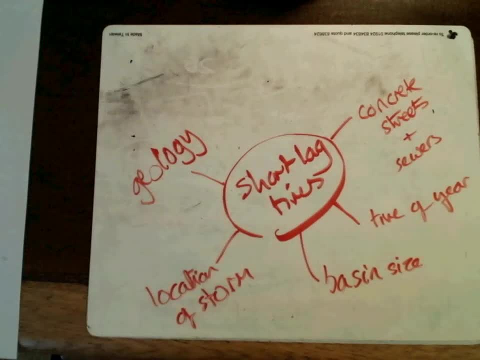 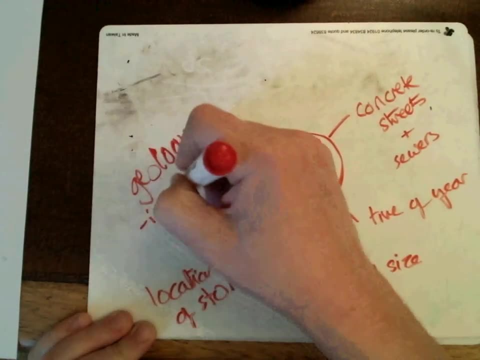 So you just need to understand that, so you just need to point out that the geology of the area may be impermeable And this means that percolation cannot take place. 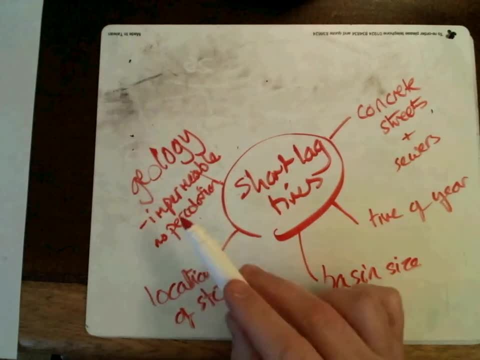 It's a slightly more complicated one, so I've added a couple of extra words there. Here are one, two, three, four, five good reasons why lag times would be short, As I said, if you check your class notes. 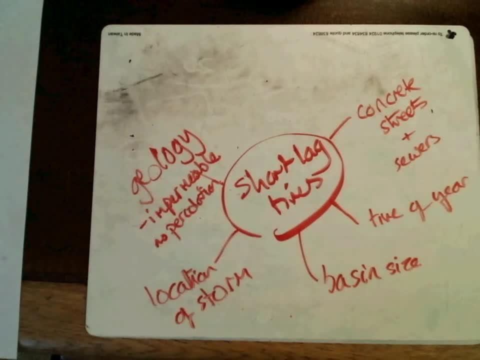 you'll find that there's actually loads. And if you look at the back of your hydrograph booklet- I think it's four pages- from the back you'll find a table that itinerizes all of the reasons. 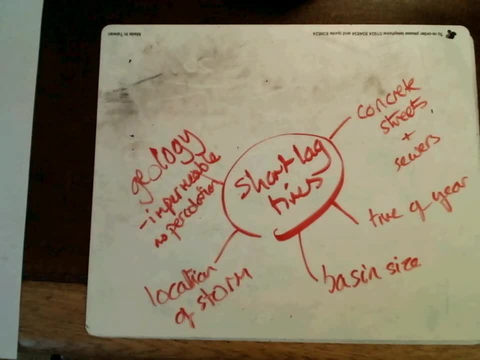 And that's a good place to go and revise. I wouldn't suggest you try and learn every single one of them. Instead, make a mind map like this and focus on the ones that you find easiest to understand. What if, though? 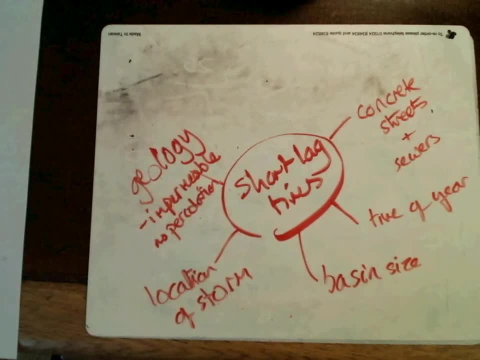 you want to describe why the river is filling up slowly, Why there is a long lag time. Well, first of all, it's worth pointing out that, of course, the basin could be a large basin. The storm could be located further away from the river. 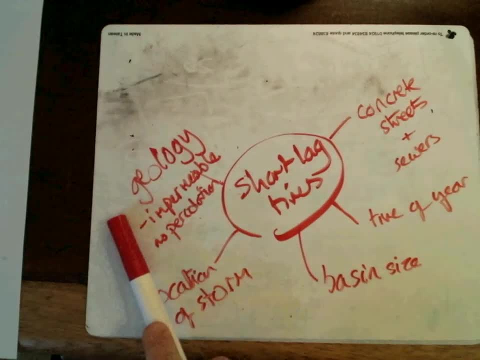 within the drainage basin. The geology might be permeable, therefore, percolation can take place And, of course, there could be an absence of urban areas, which are therefore, of course, going to mean that rain can infiltrate into the soil. 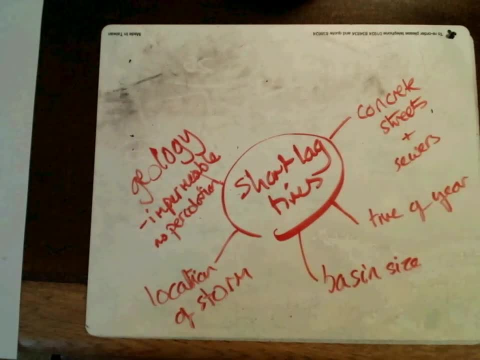 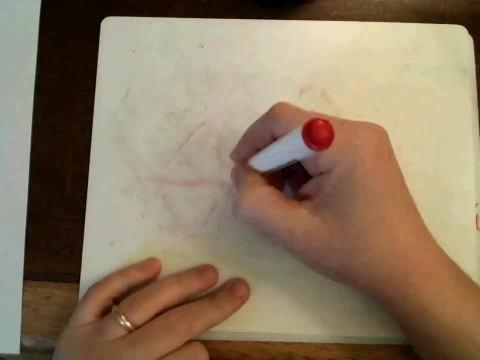 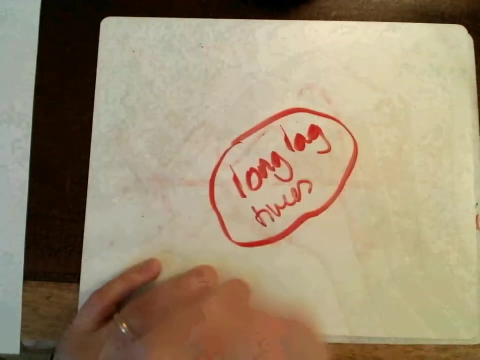 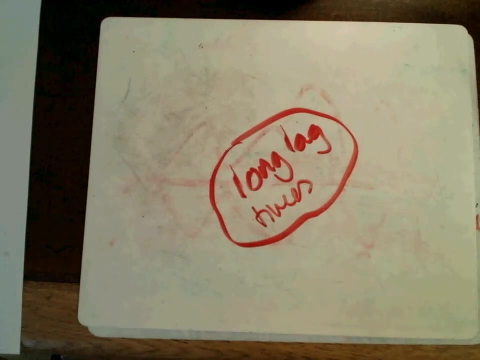 and that will slow it down. All of this is kind of obvious But just to be thorough, if we were to make a mind map of long lag reasons, there are some distinct things that most people kind of remember about long lag times. 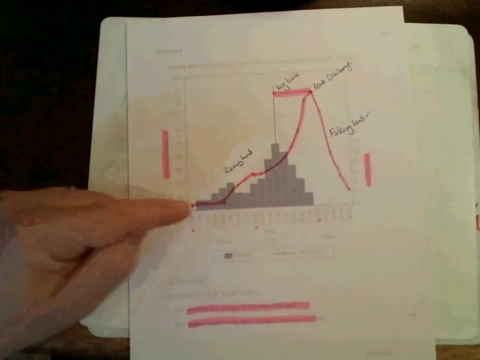 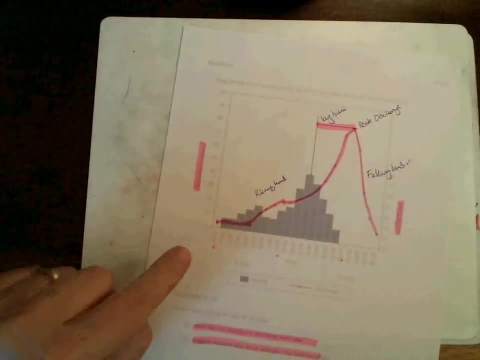 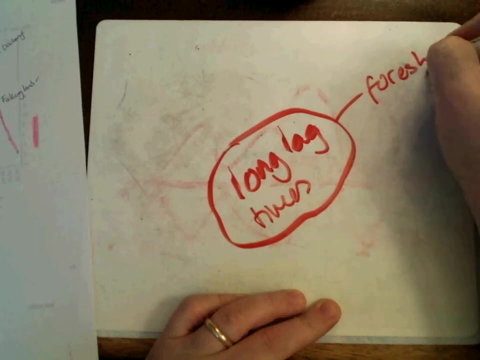 So again here on this graph, where the river is filling up more slowly, this may be because when the when the rain was falling, it was falling over a forested area, Forests and other vegetation. 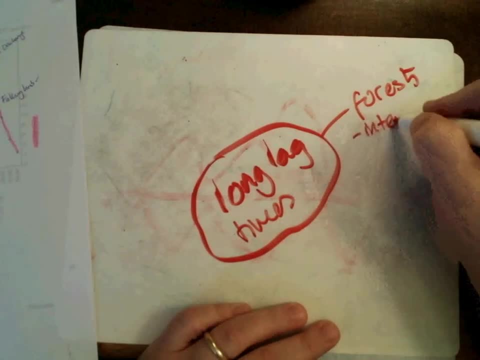 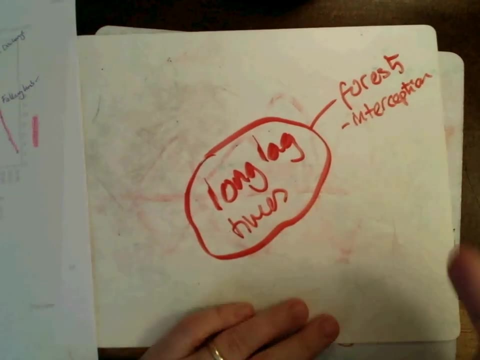 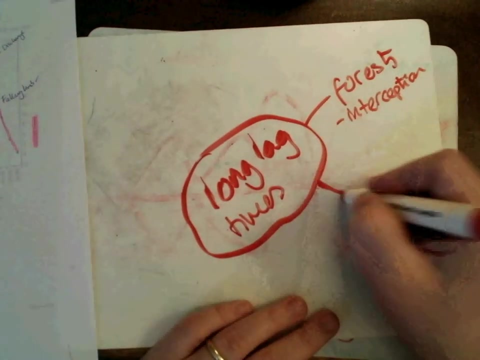 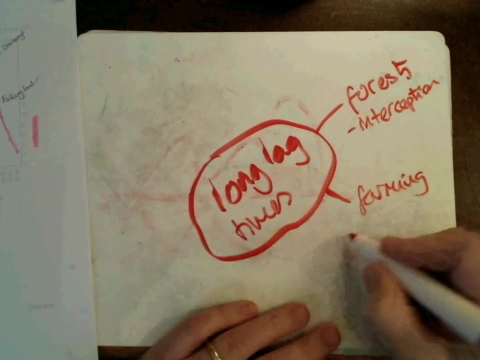 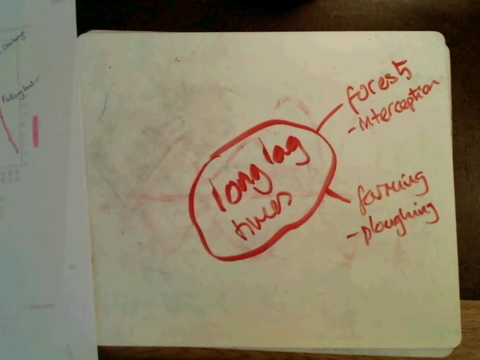 intercept rainfall. An interception slows the rainfall down in its journey across the land as surface runoff to the river. A nice, straightforward one: Farming, Specifically ploughing. Where you plough fields, you increase the pore space within the soil. 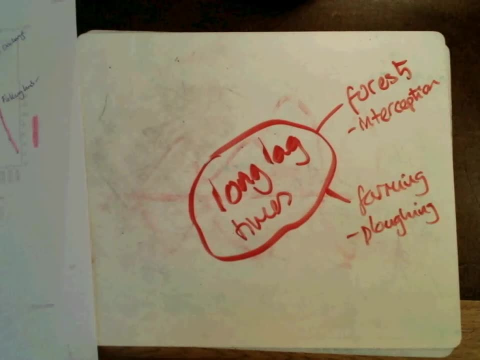 That means the gaps within the soil, and the soil is more capable of absorbing water. Also, the furrows, that's, the ridges that ploughs make in the fields. they can often slow down surface runoff on their journey across the land. 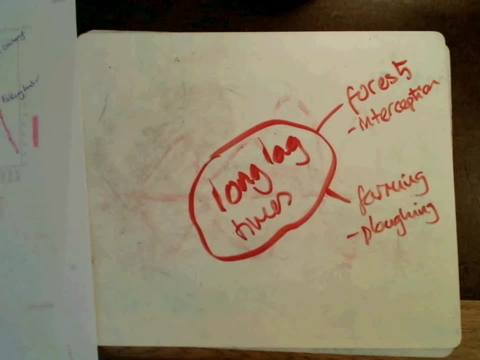 Indeed, farmers often contour plough. That means ploughing around the contours of a hill to deliberately slow the water as it flows across the land, to stop the soil being washed away. Another easy one is just. 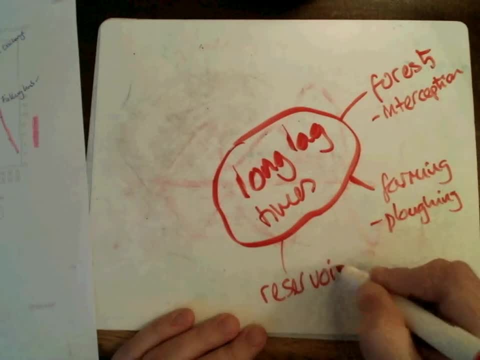 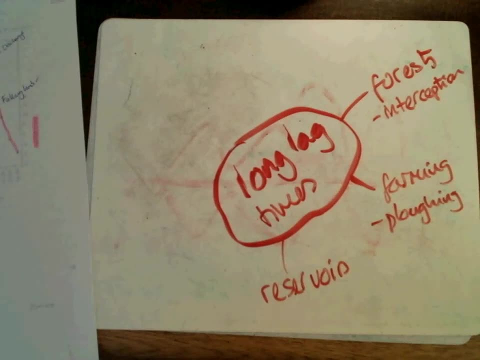 things like reservoirs. The presence of a reservoir in a river system obviously will slow down the movement of the water through the river, So the rain may be falling in one part of the drainage basin. 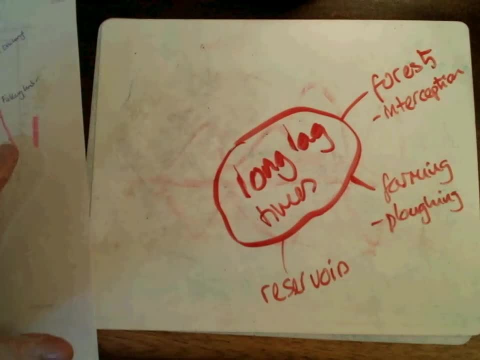 but that rain is getting into the river system and getting entrapped in a reservoir, before then making its way down the rest of the river course. That's going to slow it down quite markedly. Where else could water get stored and trapped? 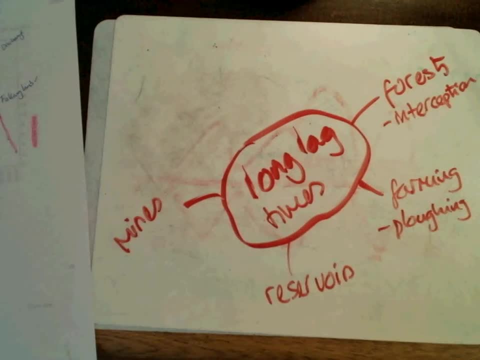 If the area is an area which involves mining- and this is West Wales, so you wouldn't need to be as specific as that- if the area is an area that has mining, then clearly underground huge holes underground. 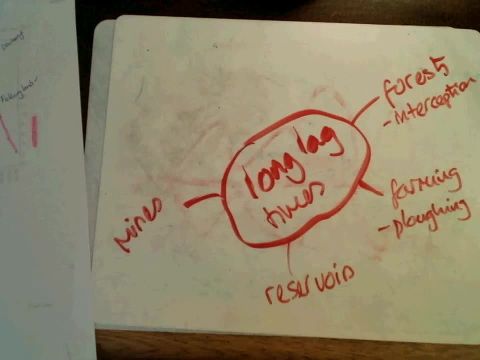 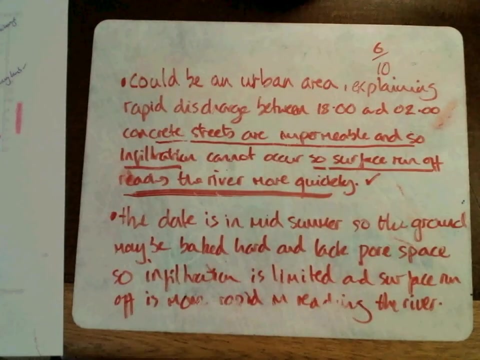 are going to be a good way for water to get stored and trapped before making its way towards the river as through-flow. So at this point in the lesson, what I've covered is what an answer needs to look like. 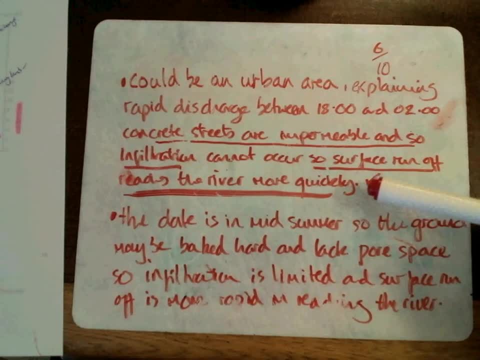 This is important. Spend some time looking at this. Think how you would express yourself, Remember, try to be detailed and try to use the technical vocabulary that we've taught you. That's what we're looking for. Notice that I am suggesting. 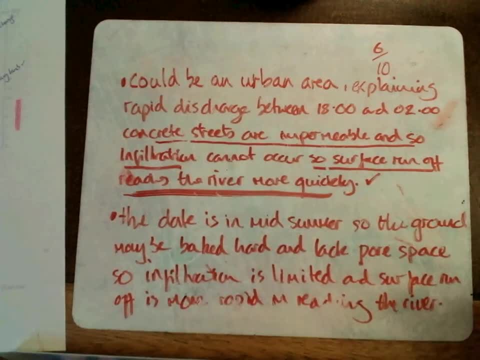 it could be an urban area. I can't deny that it could be an urban area, can I? And I'm relating that to rapid discharge. So you're being very specific. And then I've pointed out what's going to make that rapid discharge. 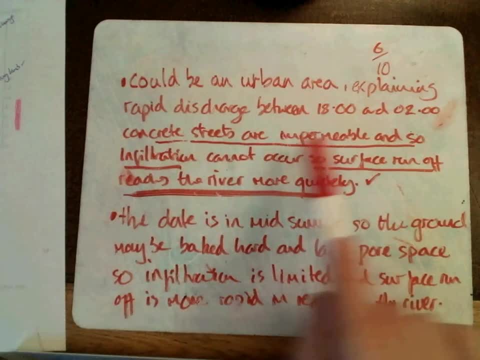 what's going to make that water travel quickly while the ground's impermeable? it cannot infiltrate, and what's the impact of that? This last bit of the sentence is important. What's the impact of what you're saying? 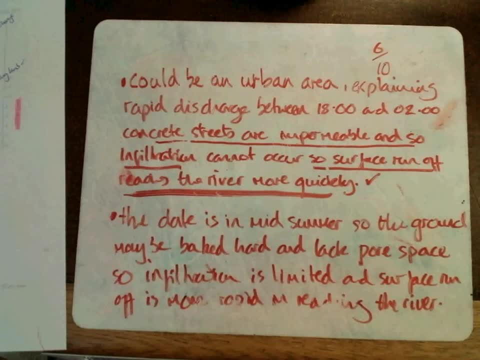 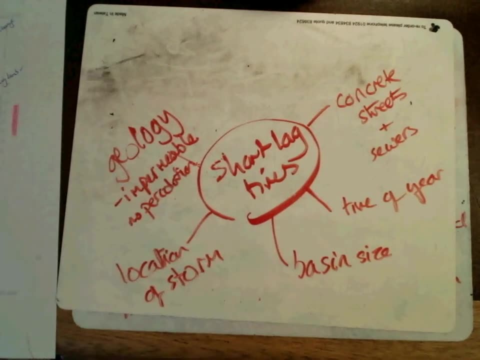 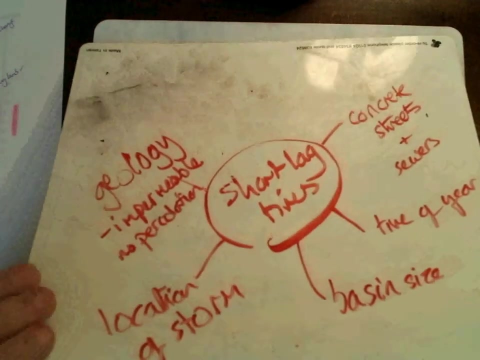 Well, it means that surface runoff is going to reach the river more quickly. We've gone through a list of possible other short lag times reasons that you could revise. Feel free to choose other ones. These are just the ones that I find. 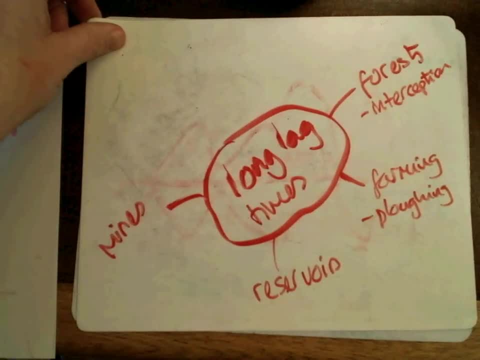 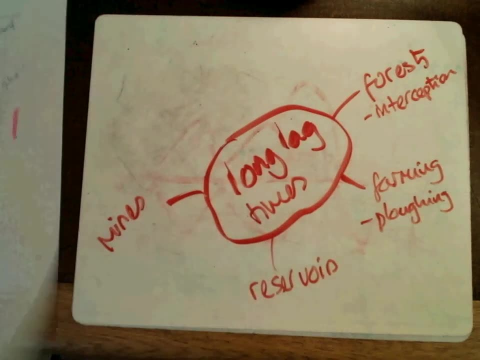 particularly memorable And also long lag time reasons. Don't try to remember every single long and short lag time reason, because it's too much Remember. this question is going to be about, I don't know, 10,, 11,, 12 marks. 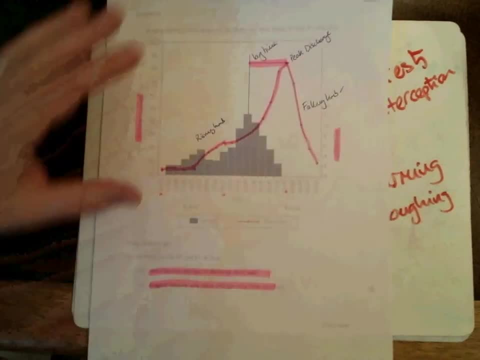 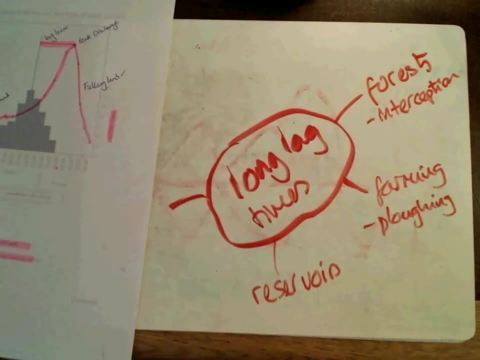 Half of those marks can be scored through description, So make sure that you're good at this bit, the describing the graph, And then you can relax a little bit about this slightly more complicated explanatory stuff. 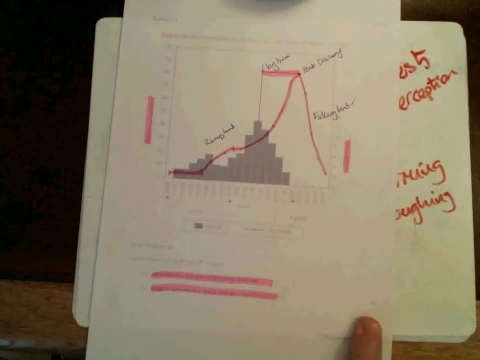 And I think you should be reasonably and quite justifiably, given that 5 out of 10. can be scored through description, you could easily be targeting 8,, 9. or even 10 out of 10.. 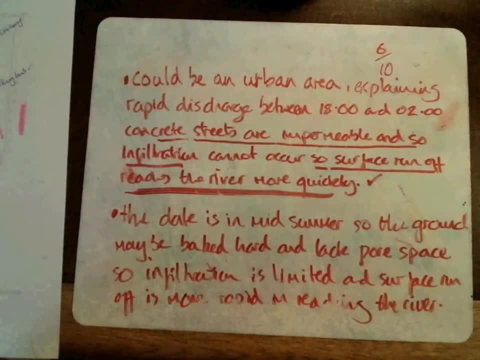 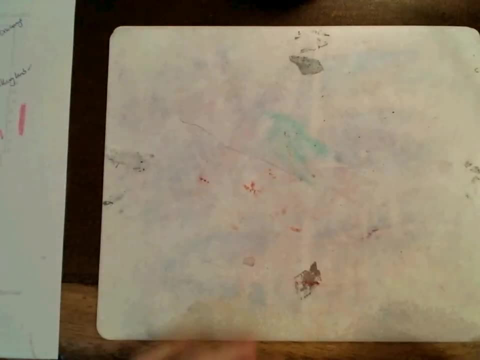 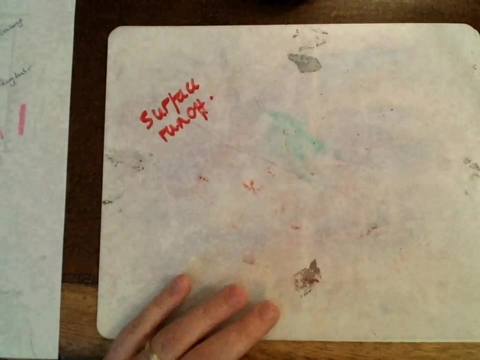 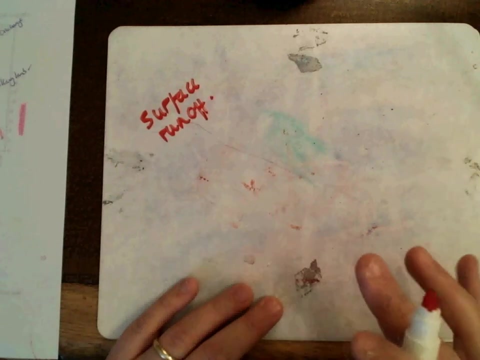 for a question like this. Okay, One last little reminder, Some key terms You need to understand: surface runoff, Surface runoff. Surface runoff is the movement of the water over land. It is sped up or slowed down according to what surface. 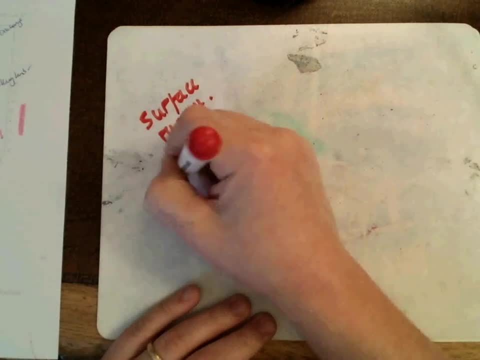 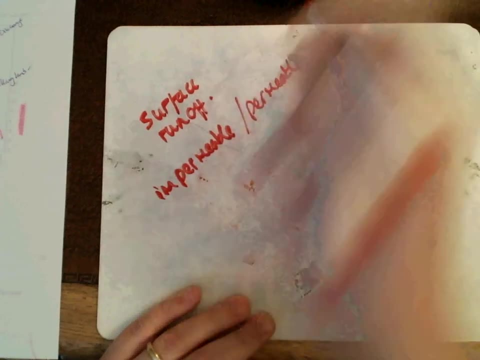 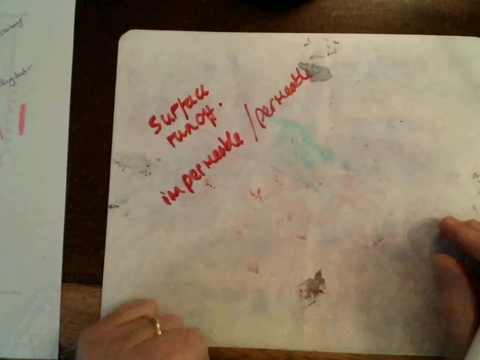 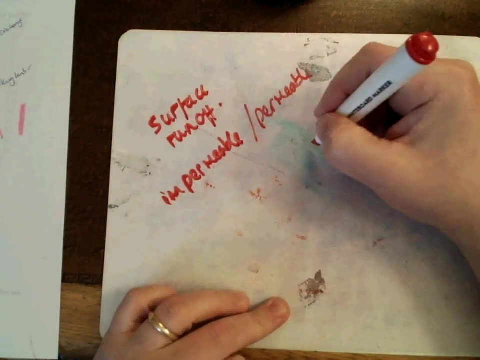 it is running off over. Is the surface impermeable or is it permeable? Concrete and rock can be impermeable, but soil can be permeable. If it's permeable, then it's going. there's going to be a process of 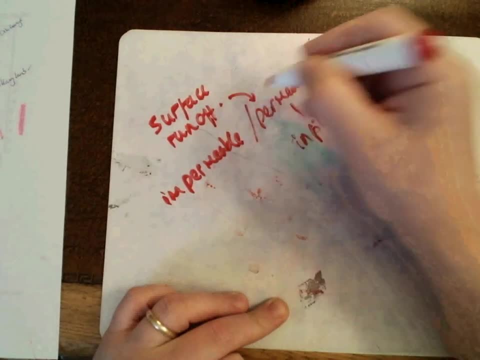 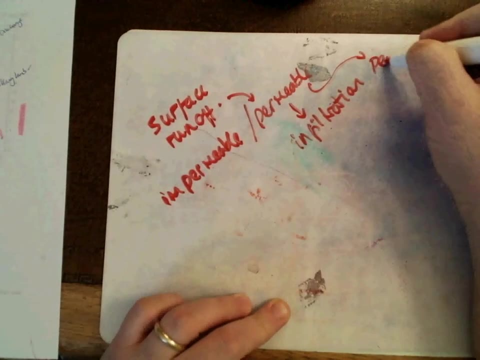 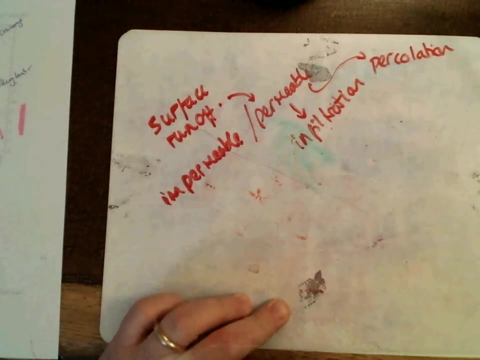 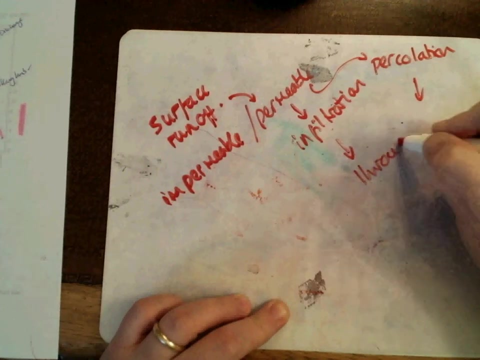 infiltration. If it's a permeable rock, this could lead to a process of percolation, Which just means dripping down through the rock. These processes will both lead to increased amounts of through flow.